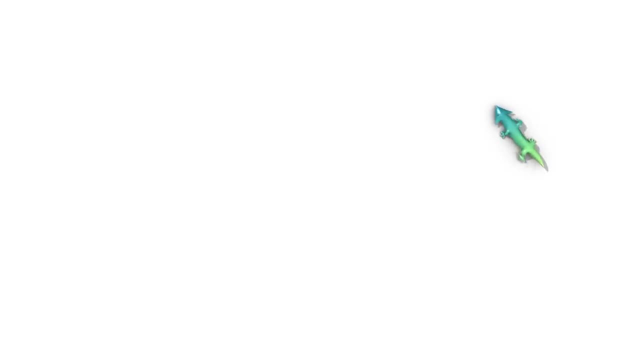 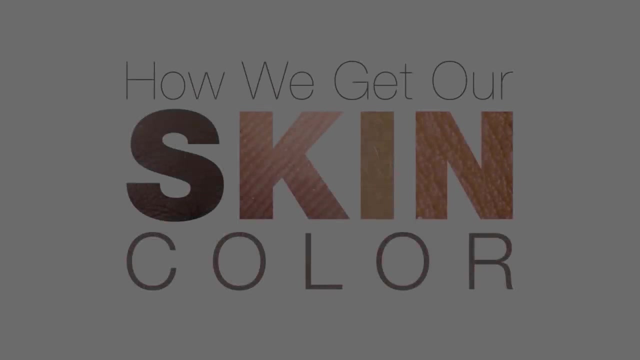 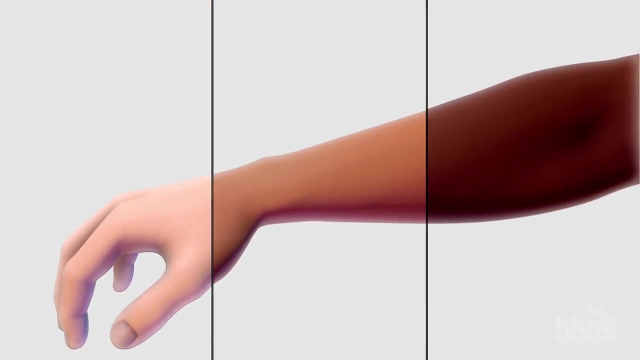 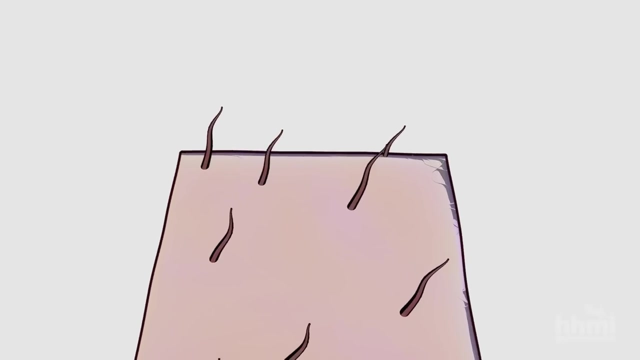 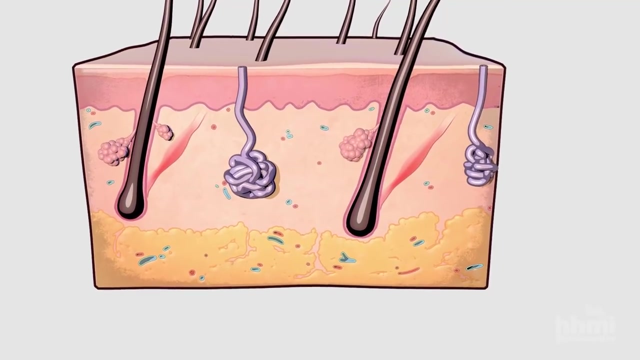 Skin covers all our bodies, but its color varies from person to person. To understand why, we need to peer inside its layers. Skin cells and their allies, hair, sweat and oil glands, form a first line of defense from the environment. 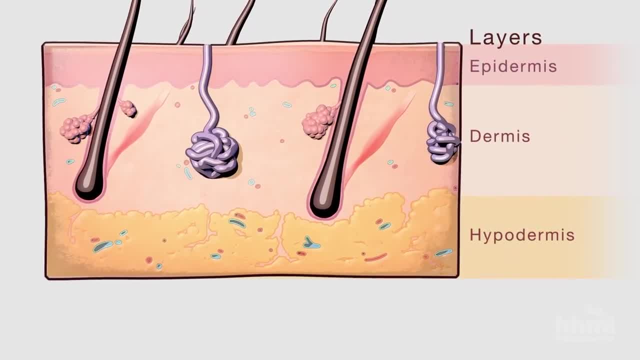 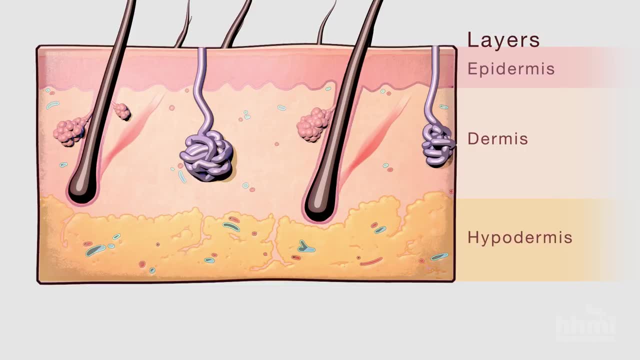 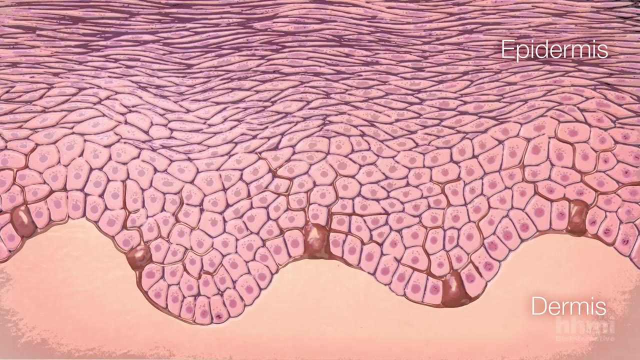 Skin's three main layers are each a distinct community of cells with different jobs. To see what gives skin its color, we need to focus on the outermost layer, The epidermis, and two important cell types: carotinocytes and melanocytes. 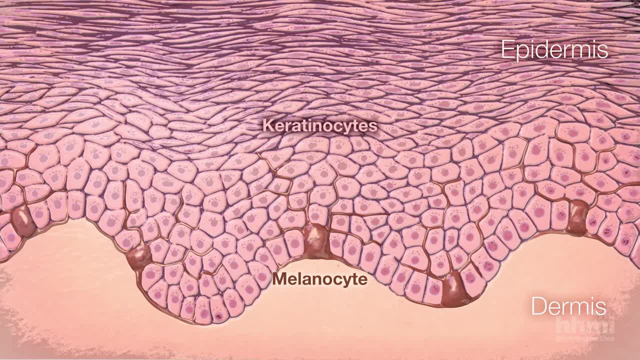 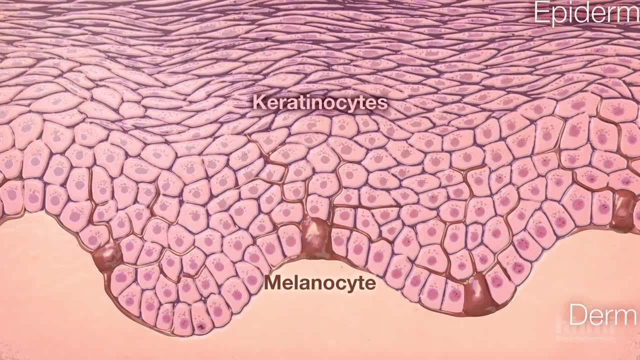 The carotinocytes are the cells that form the surface of the skin and are on the front line for taking insults from the environment. Deeper down in the epidermis, right at the base of the layer, we find the melanocytes. 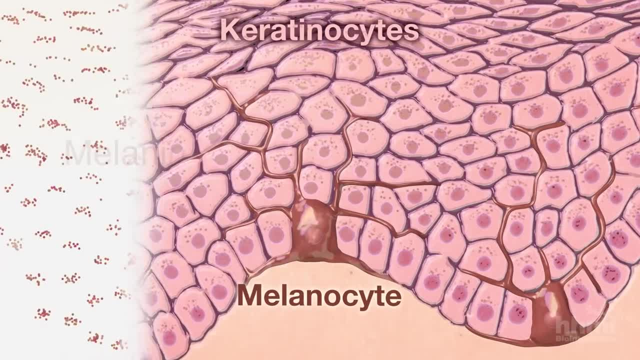 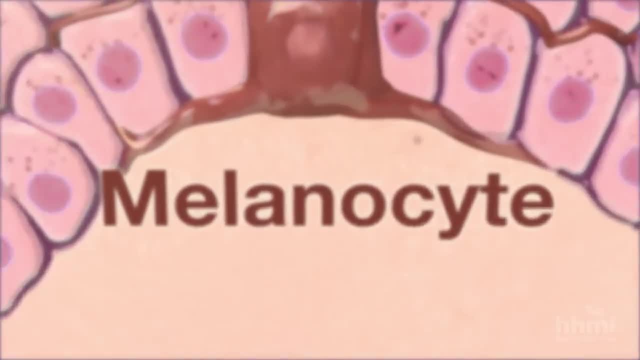 These star-shaped cells produce the important pigment melanin. The carotinocytes are the cells that form the surface of the skin and are on the front line for taking insults from the environment. Let's zoom inside a melanocyte to see how this works. 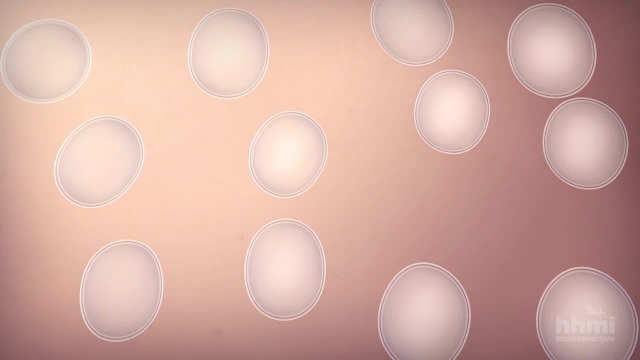 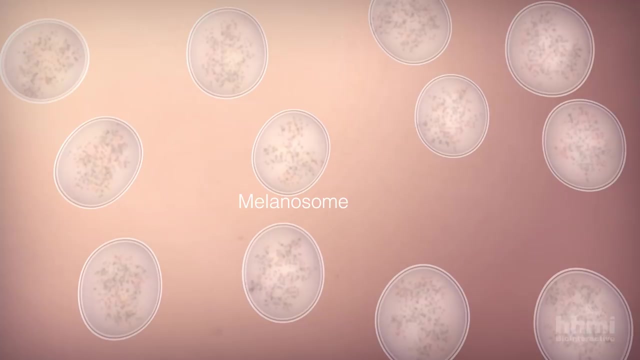 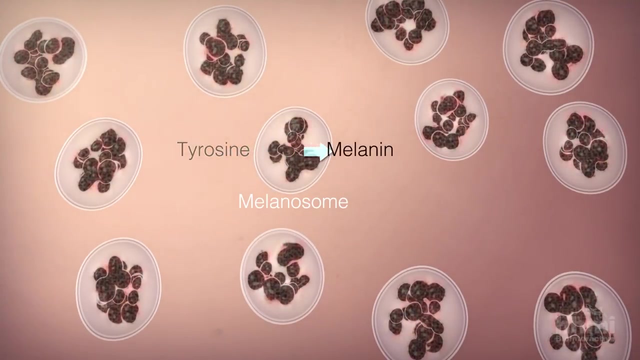 Melanin is produced inside what look like spheres throughout the melanocyte. These are the melanosomes. Chemical reactions inside melanosomes turn the amino acid tyrosine into melanin. The proportion of two main melanocytes is equal to the amount of melanocytes in a cell. 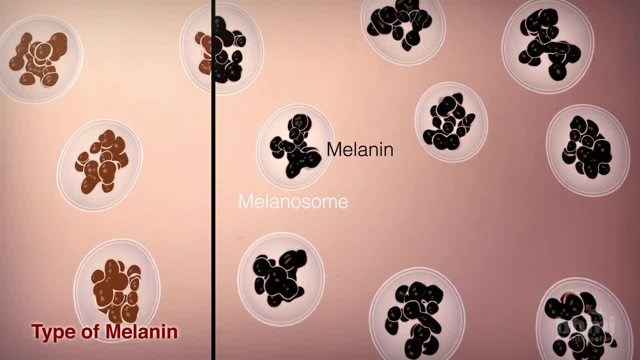 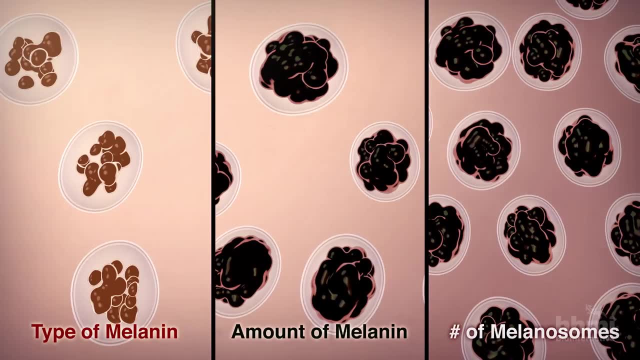 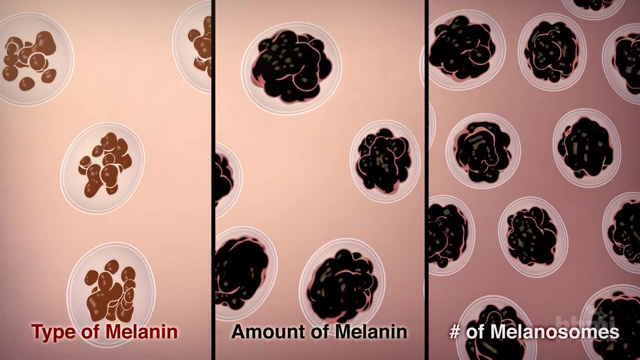 The main forms of melanin produced a reddish-yellow type versus a black-brown type. the total amount of melanin in each melanosome and the number of melanosomes in the epidermis all vary from person to person and determine their skin color. 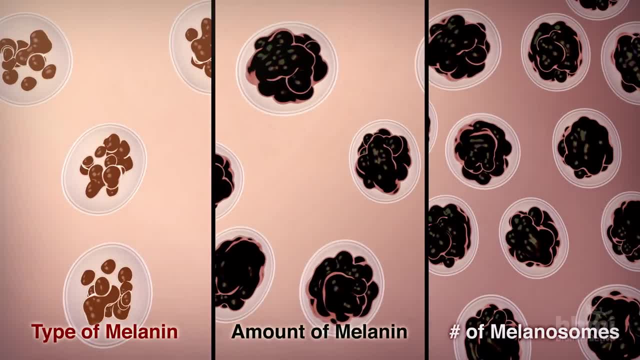 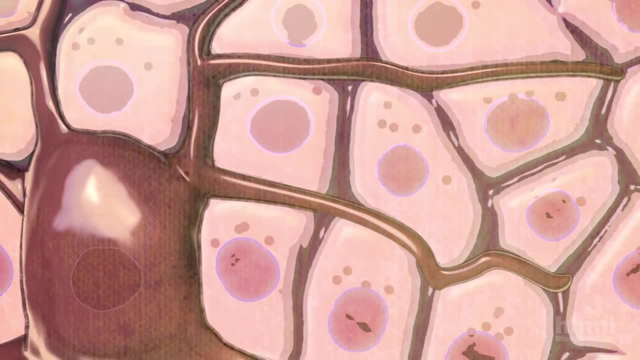 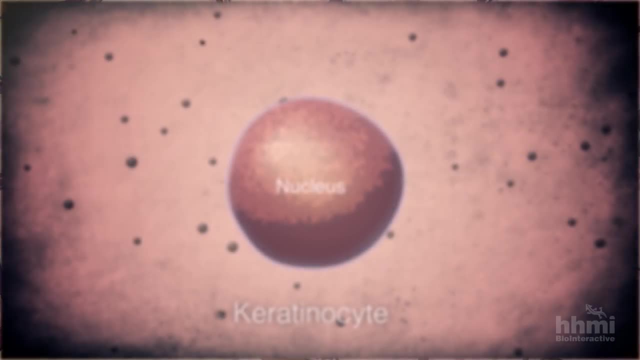 Melanosomes are the melanin factories inside melanocytes. But for melanin to do its job, melanosomes need to be transported to the carotid. Melanin is produced inside the carotid via the melanocyte's long projections.